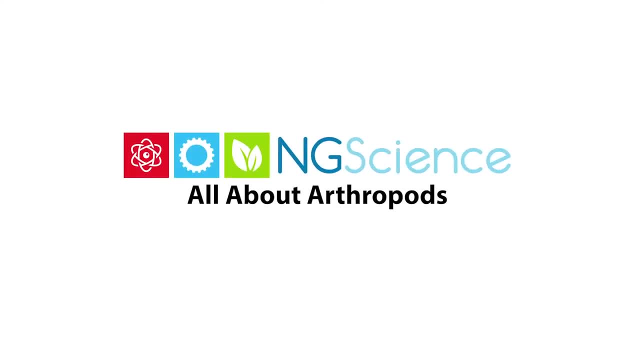 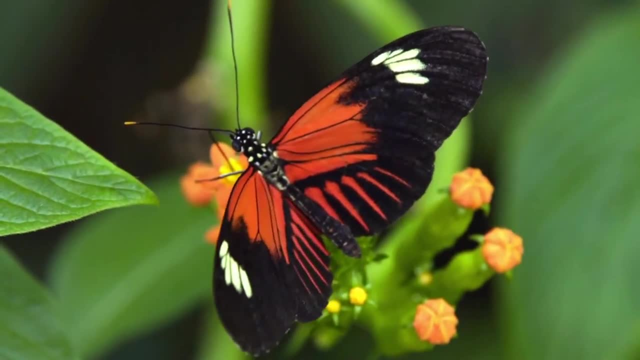 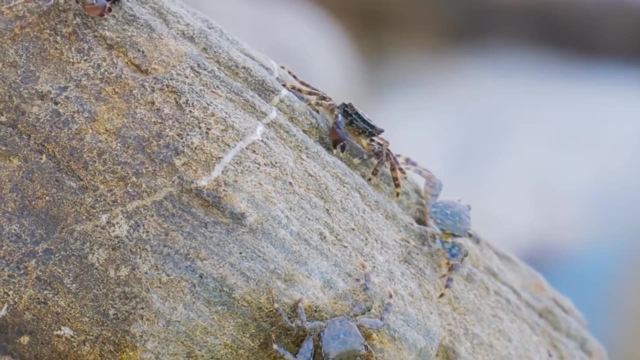 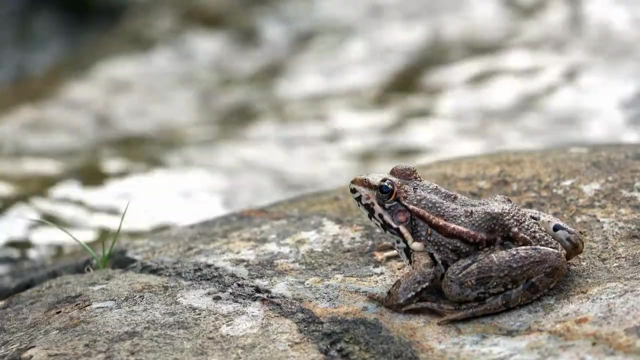 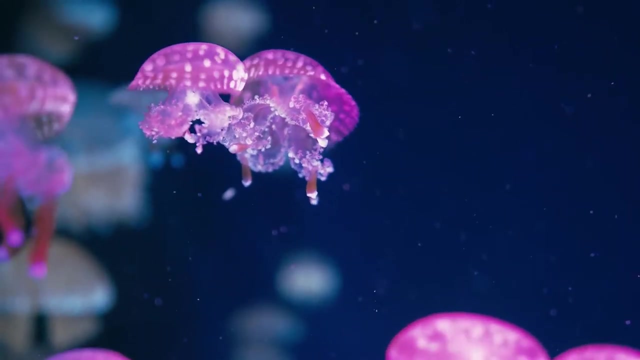 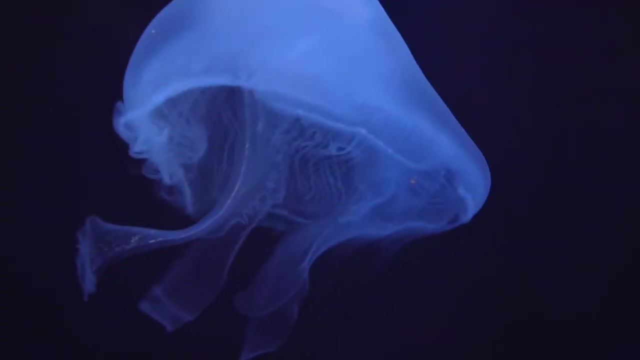 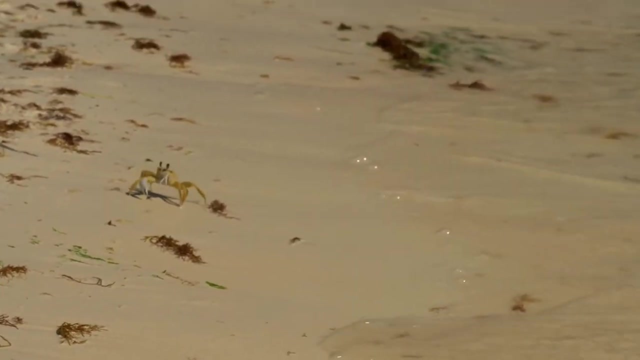 Animals are typically classified into two main groups: vertebrates, which are animals with a backbone, such as mammals, birds and reptiles, and invertebrates, which are animals without a backbone, like insects, spiders, worms and jellies. today, we're going to take a closer look at a fascinating group of invertebrate animals- arthropods. arthropods are the most 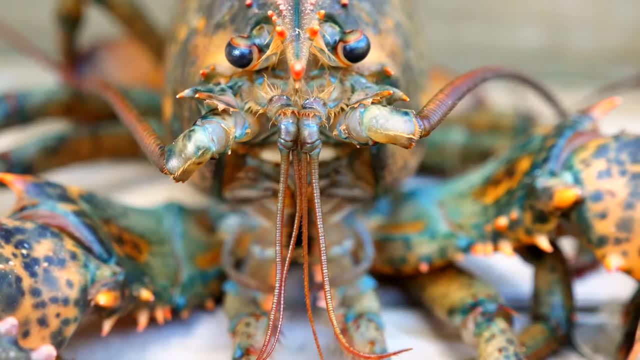 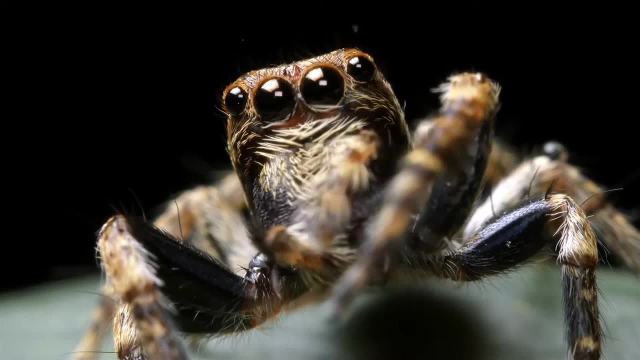 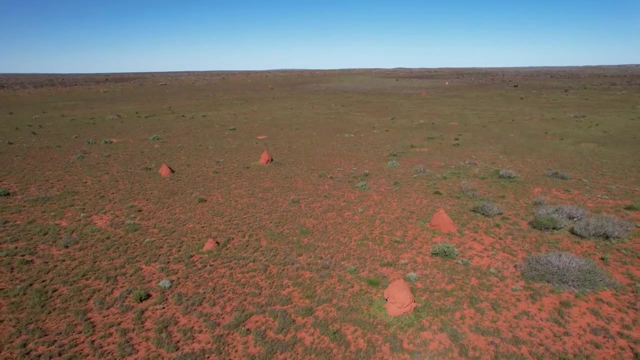 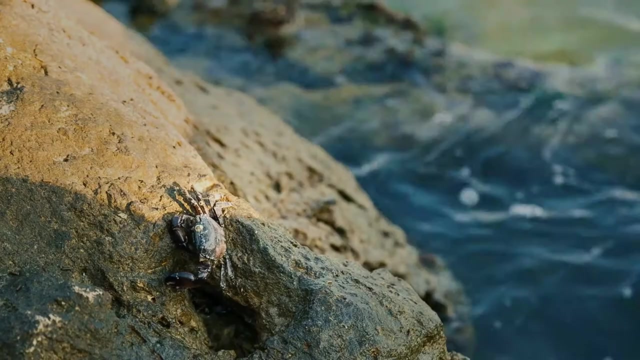 diverse and numerous group of animals. they make up over 80% of all known species of animals. they live in all areas of the earth, from the deep ocean to hot, dry deserts and moist tropical rainforests. common aquatic arthropods include crustaceans such as crabs, shrimp and lobsters, and 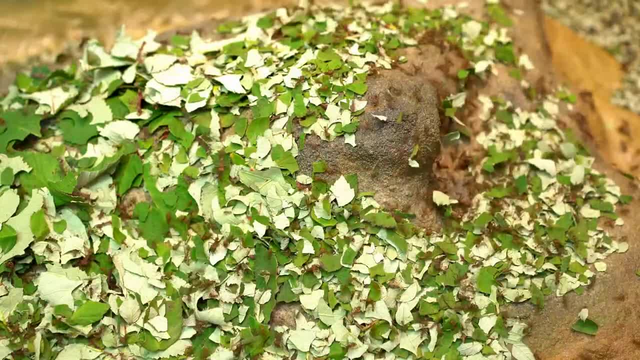 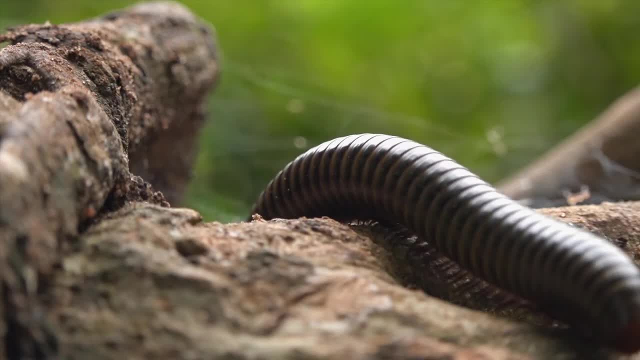 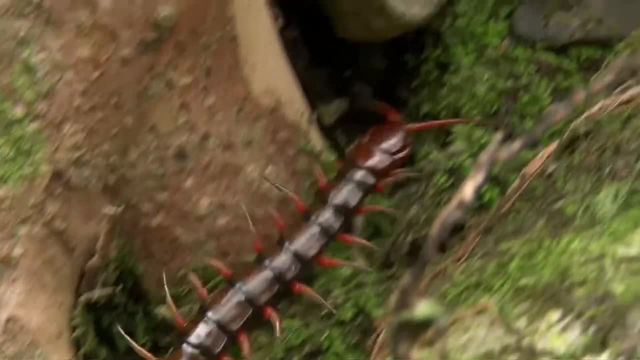 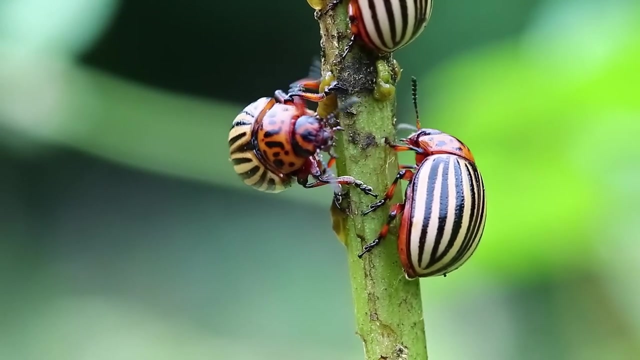 terrestrial arthropods include insects, spiders, ticks and millipedes. arthropods have a hard outer body covering called an exoskeleton made of cotton. the exoskeleton supports and protects the animal's body and can also help reduce water loss in order to keep growing arthropods. 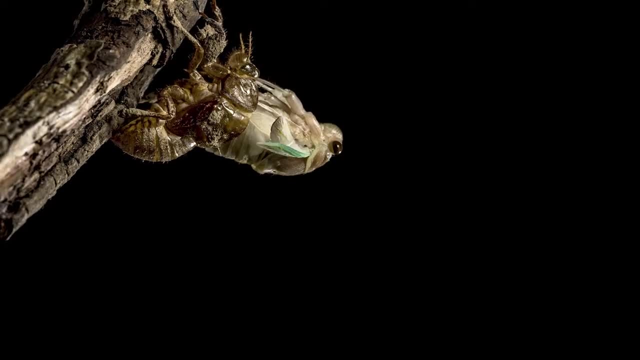 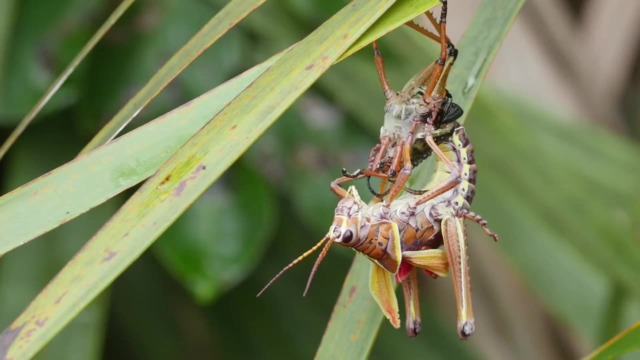 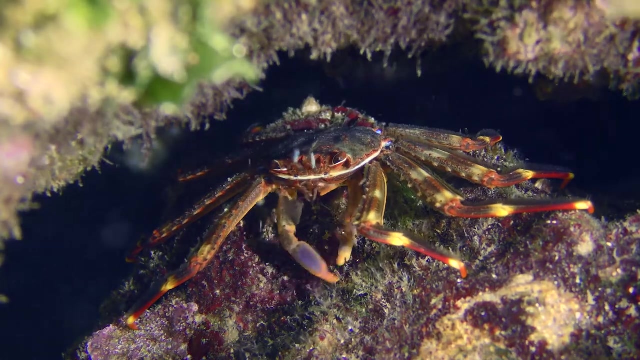 go through stages of molting, a process by which they shed their exoskeleton and grow a new one without an internal skeleton to support their bodies. arthropods are usually small in size. aquatic arthropods, such as crabs and lobsters, are often larger than land.